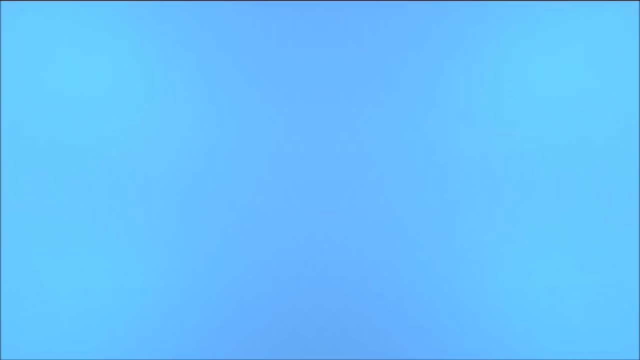 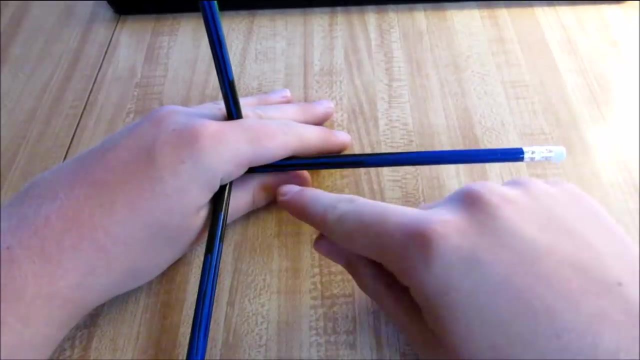 We hear it all the time that our world is three-dimensional. It makes sense, after all. We can only define up to three directions, each at a right angle to each other, that don't interact with each other. No matter how far left or right you go, you won't move. 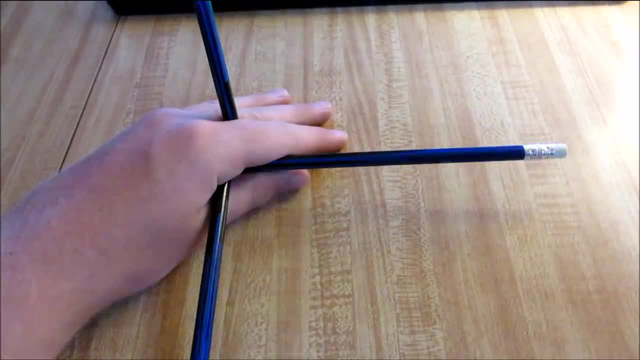 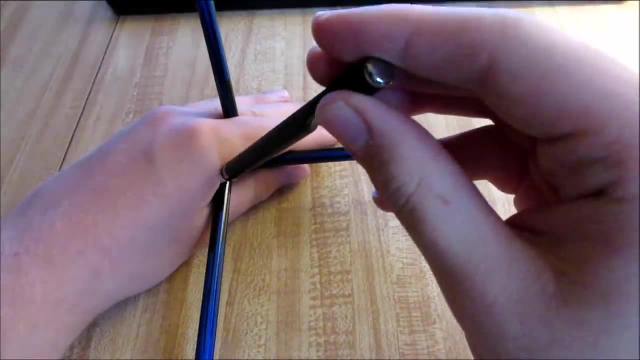 up at all, But the moment we try to add another dimension into the mix, it all breaks down. No matter how hard you try, in our three-dimensional universe you can't lay out four or more directions that won't interact. Now I know what some people are thinking. Can we consider time? 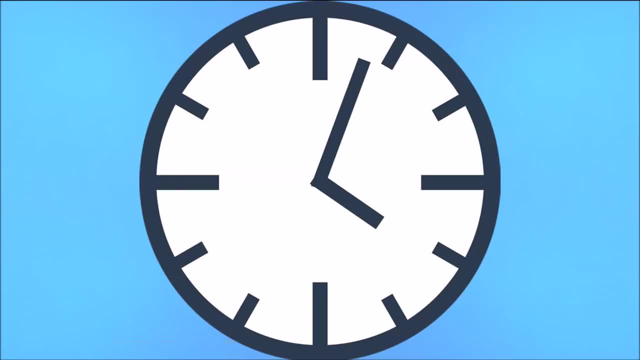 a dimension. In simple terms, it does make sense. We can measure time and tell one point in time from another in a linear sense: Four hours later is always four hours later, just like how four feet to the left is always four feet to the left. Heck, you could even make. 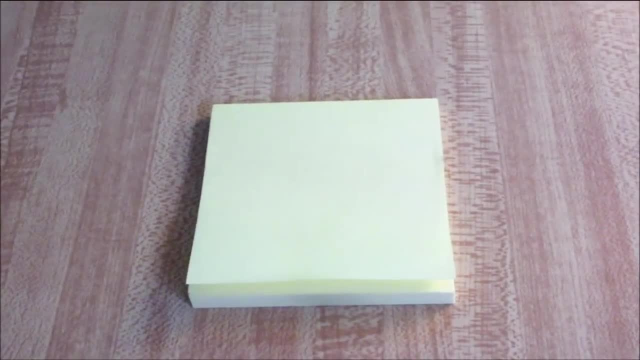 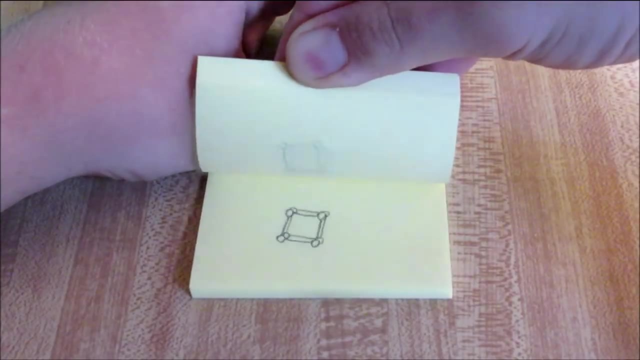 time act like a spatial dimension. Take a flipbook: Each frame of animation is a two-dimensional image, but by traveling through the 3D stack of these two-dimensional frames at a consistent rate, we can make time act like a spatial dimension, where height in the stack of 2D 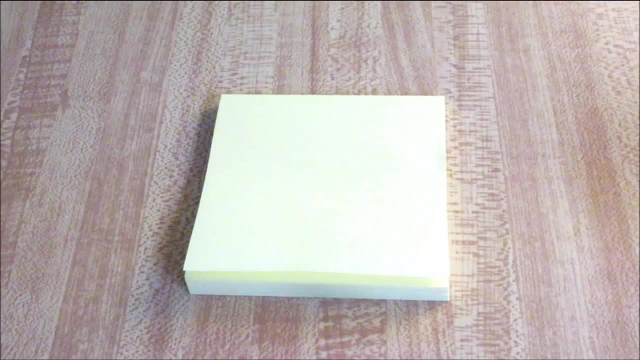 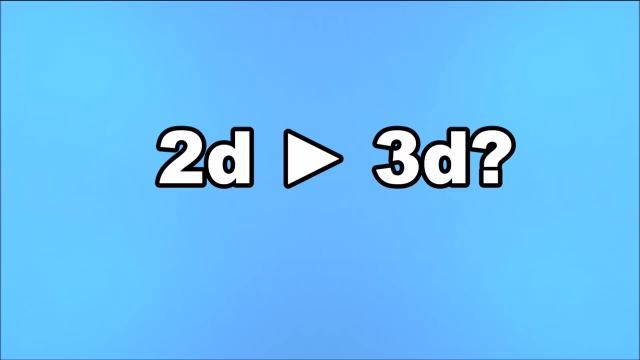 frames is the same as time between frames. In that sense, this 2D animation just became 3D right, Not necessarily. Just because time can match up with a spatial dimension doesn't mean that it is one. Notice how in the animation. 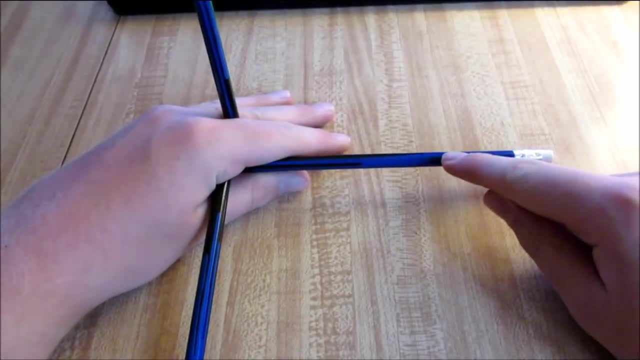 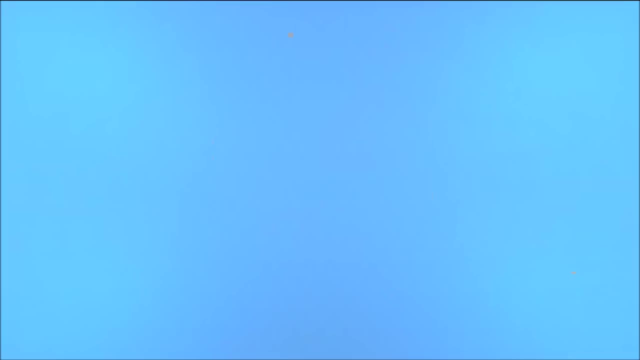 time only moves one way, from the bottom of the stack to the top, but in regular 3D space one can move either way up or down. This doesn't mean it's wrong to imagine time as a spatial dimension, since it clearly can be done, but rather it's wrong to assume a. 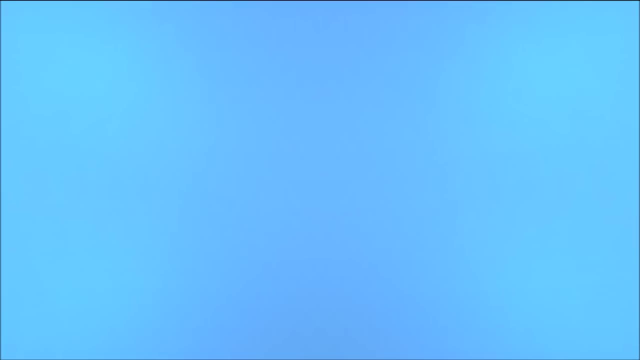 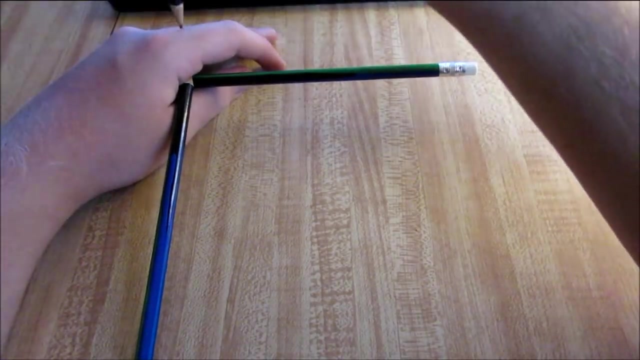 spatial dimension and time are exactly the same. So now that that's clear, let's move on to the next step. The easiest way to answer that question is actually to do the opposite. Rather than add a dimension in, let's take a dimension out. 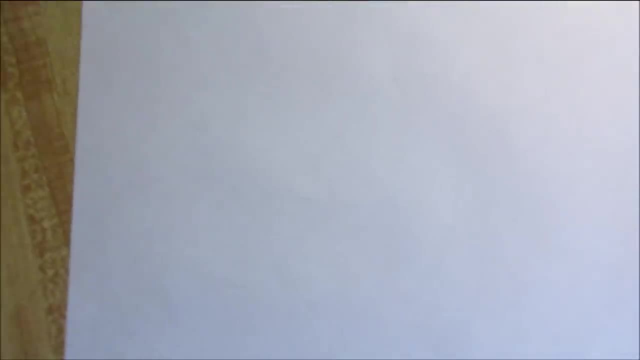 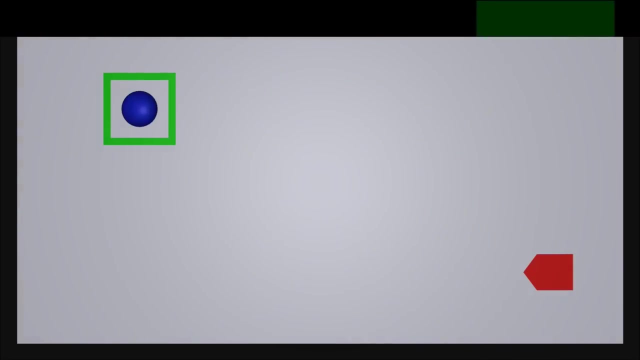 Try to picture what it would be like to live on the surface of a sheet of paper. You can no longer jump up or down off the paper, because up and down don't exist to you anymore. You can't look up off the paper either. All you can do is look forward across the paper. When 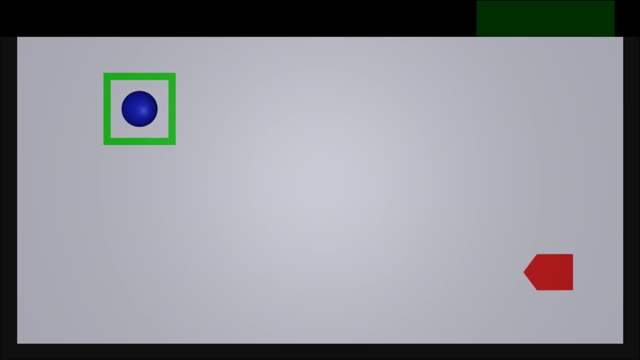 you do look in front of you, you'll see a horizontal line and in that line you'll see the edges of other 3D frames. Imagine a circle in a box. Clearly to us as 3D beings, we can see the circle in the. 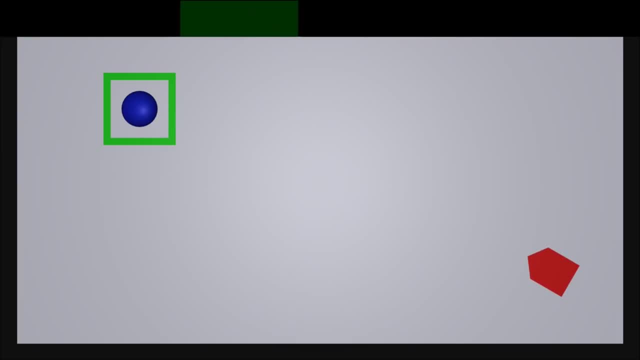 box but to a 2D, being the size of the box, would prevent anyone from seeing inside. Also, consider that whenever something casts a shadow onto, say, a wall, the shadow forms a line on the wall. Of course, to you all the walls would be lines anyways, so you wouldn't really. 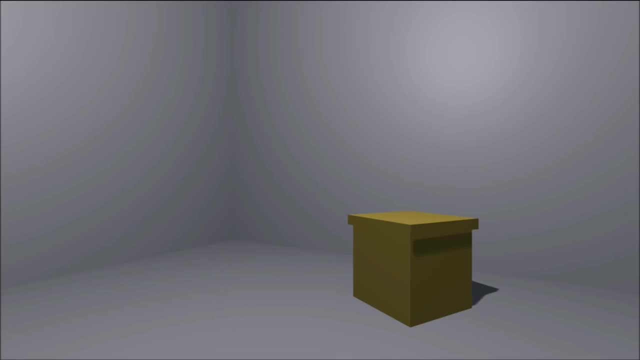 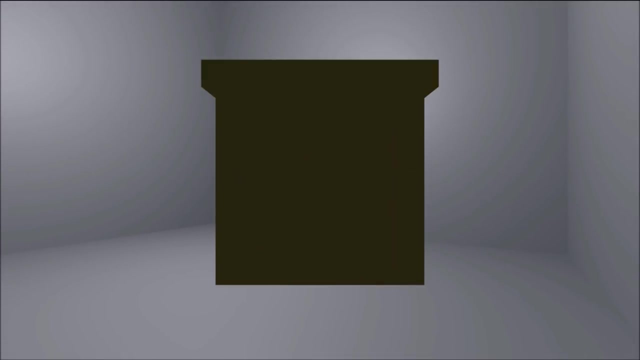 notice. Let's bring that same situation into 3D. As you look around, all you can see are 2D objects, Just like how even the box in two dimensions looked like nothing more than a line, Since you can only view it from one side at a time: the front of the box in three dimensions only. 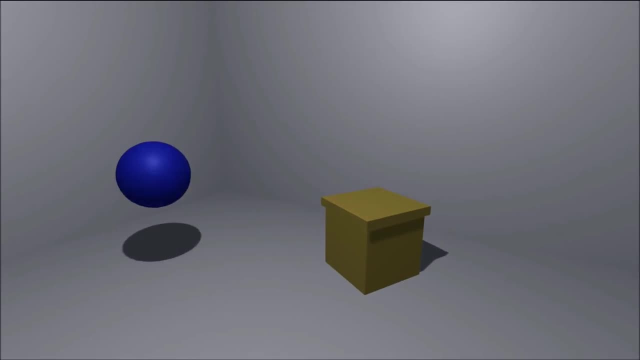 looks like a square. Also, suppose the ball was still in the box, but now it's a sphere inside a cubic box. We still can't see it now because all of the sides are still covered. The shadow the box casts on the wall looks different, Instead of just being a line like. 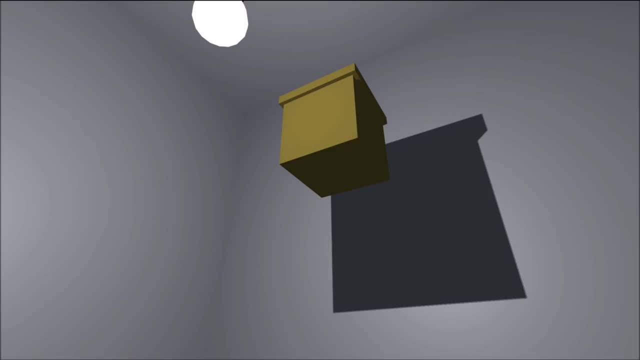 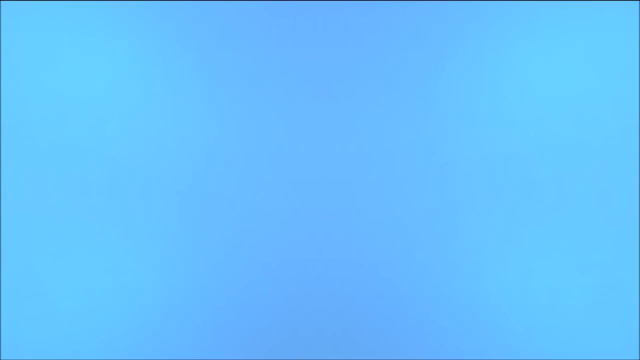 before now. it's a flat 2D shape. If you wanted, you could even trace it onto paper and get 2D drawing out of it. Here's where things get tricky. Let's try to add a new dimension that we haven't ever. 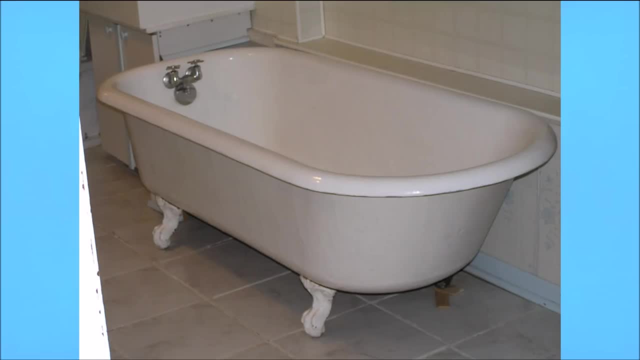 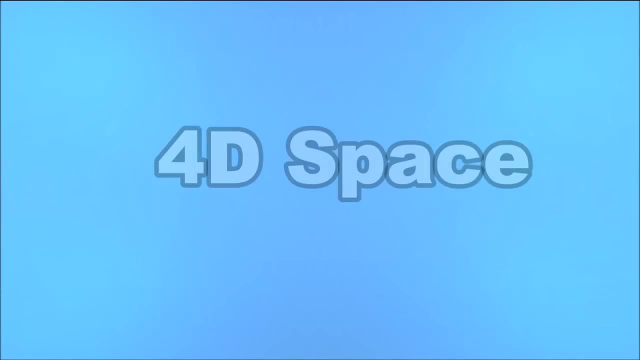 seen before. Let's just dip our toe into the four-dimensional water and use the differences between 2D and 3D space to determine what would happen in 4D space. One of the first things you would notice if you looked in a 4D space is that you would see the world as 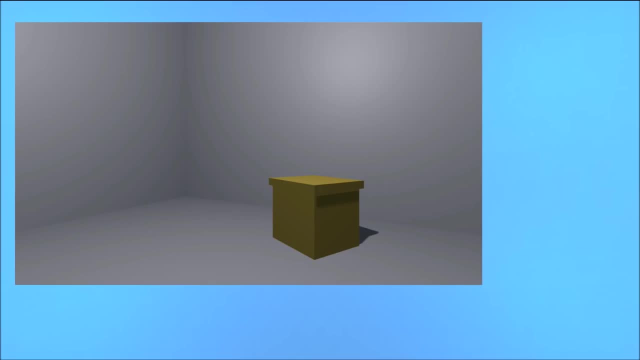 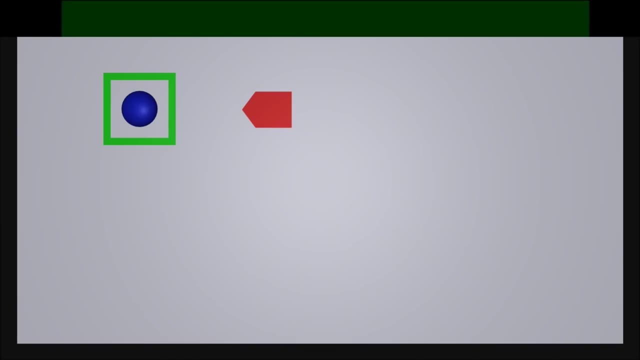 a 3D shape in a similar way to how you view a 3D world and can put it onto a 2D picture. But there's one catch: You can see all the sides of a shape. If you were to put a circle in a 2D box, you could still see it looking down from above. 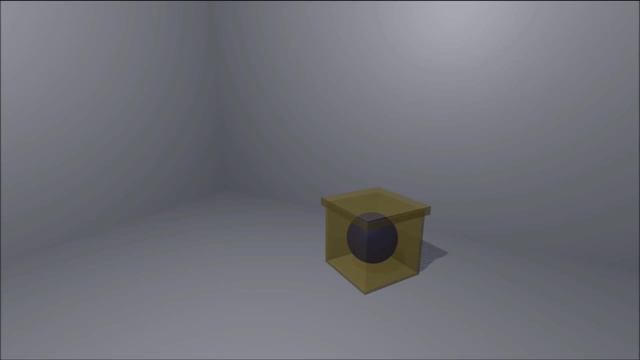 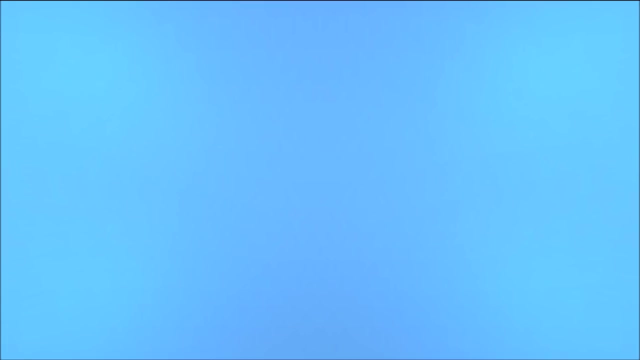 in 3D. Well, now in 4D you can see every side of the 3D box when looking down on it, including seeing the ball inside. Are you freaked out? yet After you get over the bit of wonder you experience being able to see inside of the box, you might also notice that another 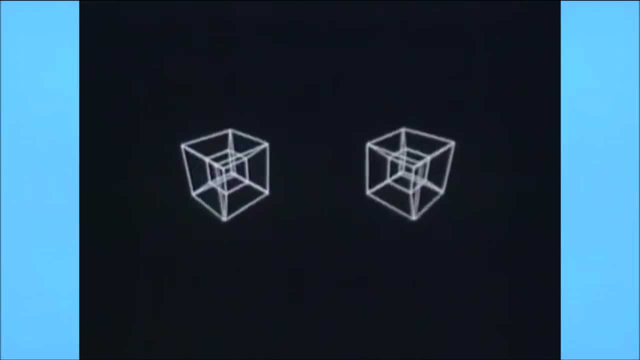 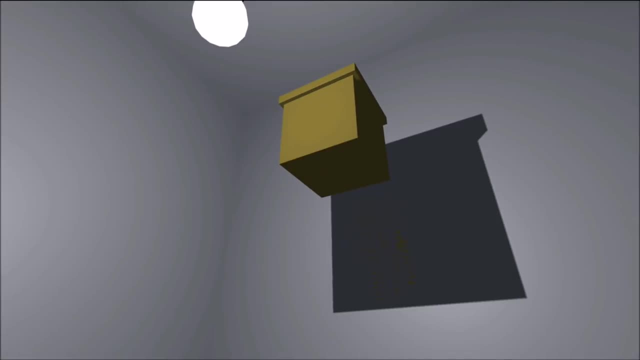 4D box is casting a shadow on the wall And the shadow… it's a 3D shape. Yes, just like how 2D space has linear shadows, 3D space has 2D shapes. Here in 4D space we have three-dimensional shadows. What would one of these shadows look? 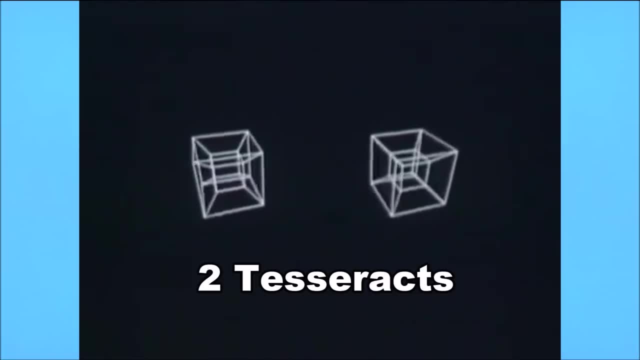 like. Here's an example. This is called a tesseract, which is the shadow you would get from casting light through a 4D cube. Notice how it's made of two cubes connected at the vertices, just like how you can draw a cube on paper from two squares and connecting. 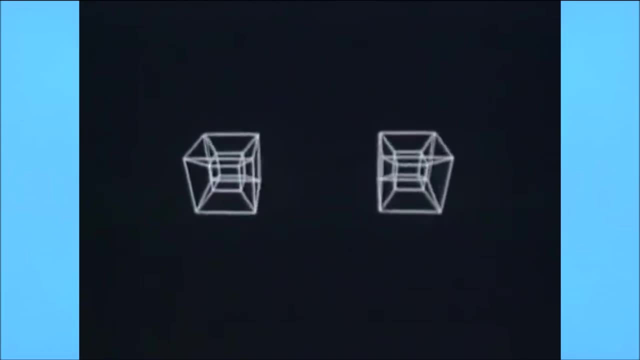 the corners. Now the tesseract looks weird enough sitting still, but watch what happens the moment you start rotating it. I'll give you a moment to clean up your mind, which most likely at this point exploded. Yes, that's what the shadow of a 4D cube looks like when. 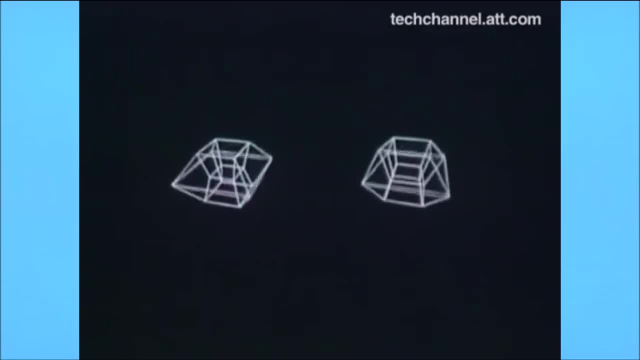 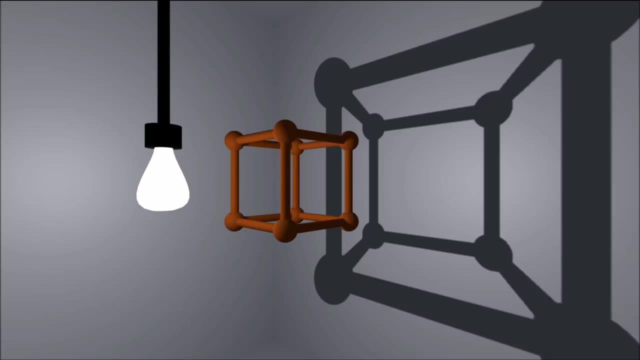 the cube rotates. Why does it do this where the middle cube stretches out to become the outer cube? Let's take a look at the shadow of a 3D cube. First note the two squares. One is smaller than the other because of perspective, making further objects appear smaller. But 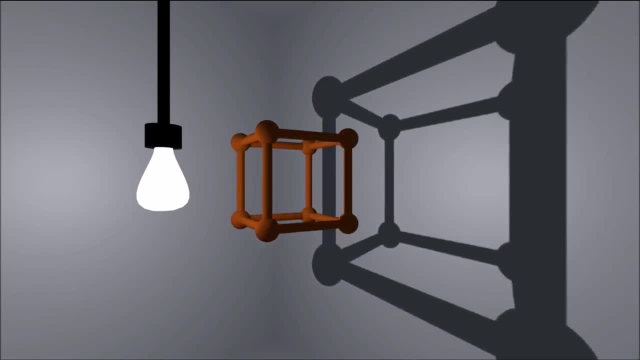 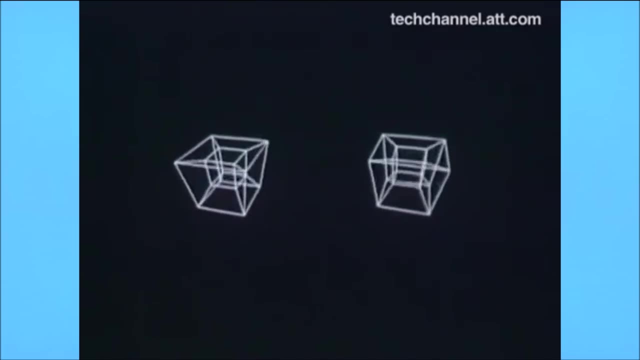 if you follow the small square, you'll see that it moves to the other side before eventually moving to the front of the cube and becoming the big square. Now watch the tesseract again. Because of 4D perspective, when rotated to be closer it becomes bigger, while the big 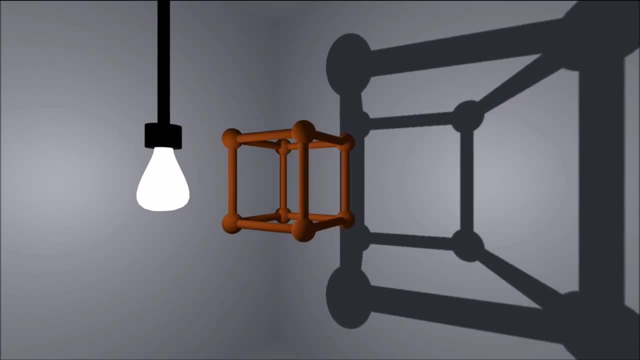 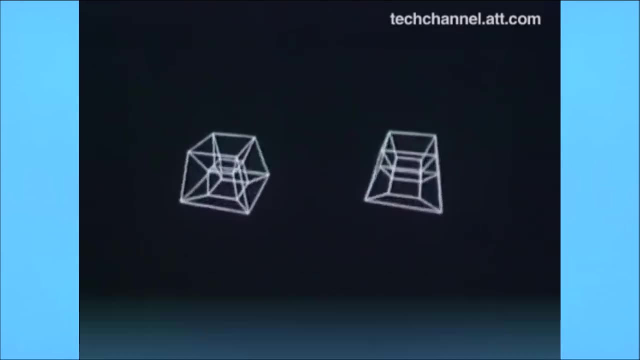 cube rotates to be smaller. So, just like in a 3D cube, where the big and little squares switch places, in a 4D cube the big and little cubes will switch places. All in all, four-dimensional space isn't all that bad, In fact, with the proper understanding. 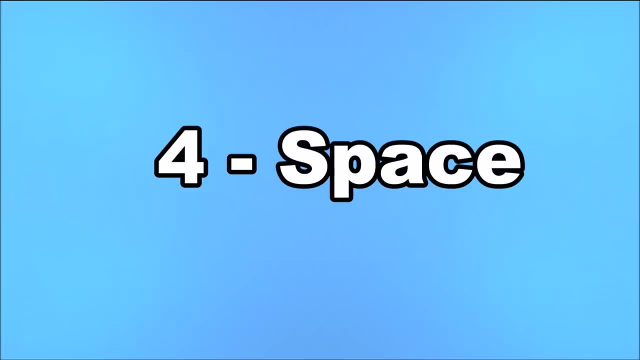 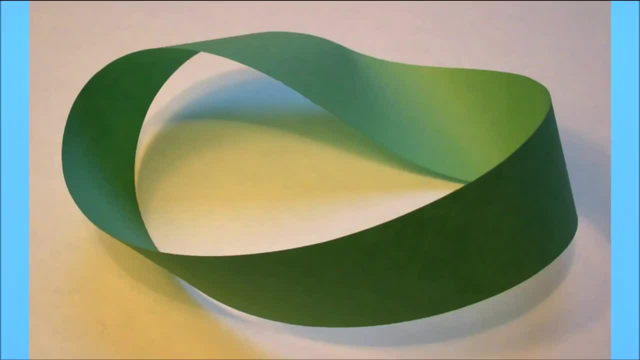 of what will happen. one can devise some clever shapes that do things we can't even imagine doing in 3D space. Ever hear of a Mobius strip? It's a plane that, thanks to its shape, can be bent around in 3D space and has only one side, because what would normally be the 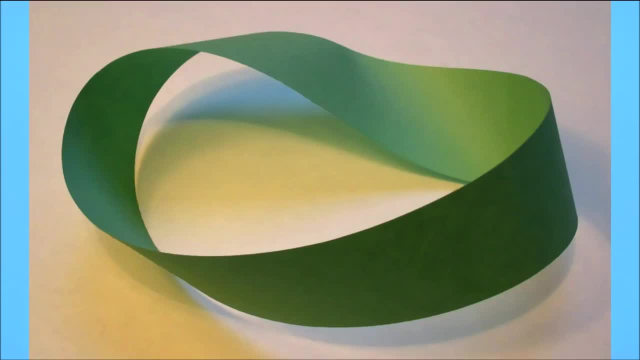 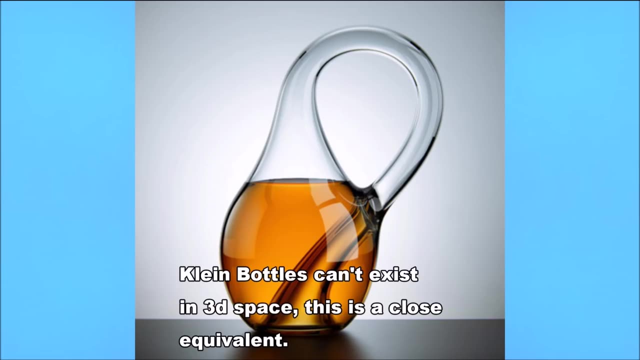 top and bottom sides are now connected, making them the same. Thanks to a little 4D trickery, a figure called a Klein bottle can exist where the inside and outside are the same. Ever notice how you can mirror writing on a page by flipping it over In 4D space? you?